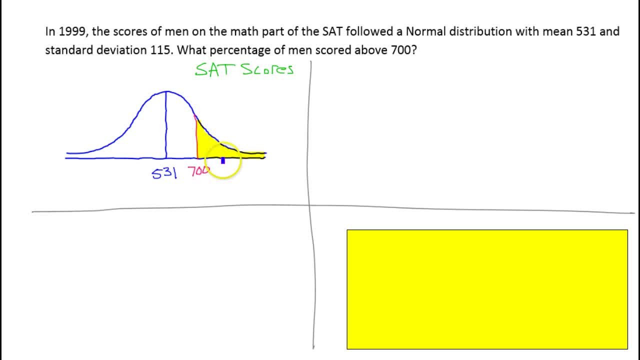 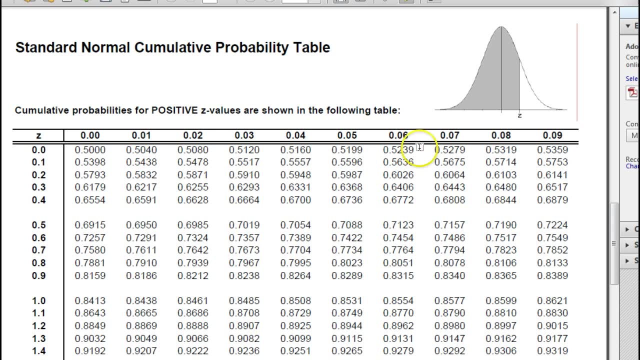 percentage of values to the right of 700 on this graph. Okay, a z-score chart like this tells us the percentage of data that is to the left of any z-score, Any z-score you want. the chart tells you what percentage of the data. 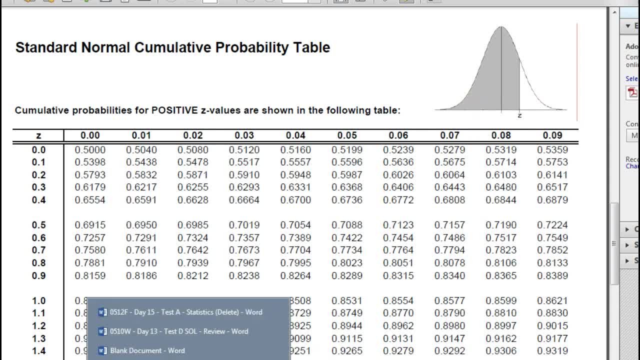 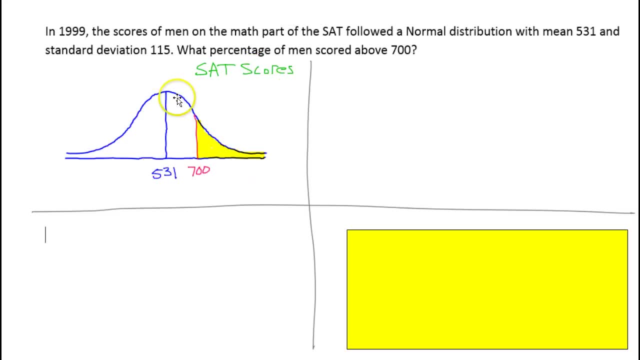 is to the left of it Now. so first of all we need: this is all based on z-scores, not SAT scores. So that's fine, because we know a formula to convert from SAT scores to z-scores, And I'm going to draw a picture of that over here on the right-hand side. So this: 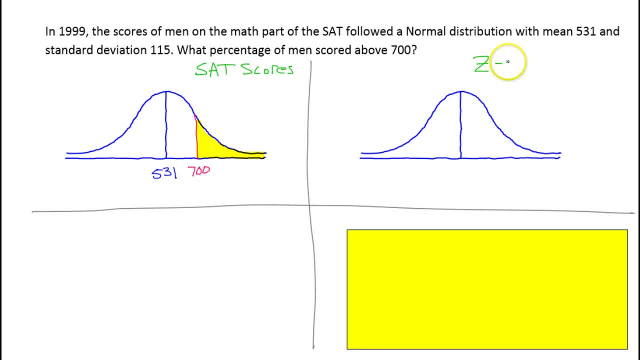 graph is going to be a graph now of z-scores. Alright, so we can really understand the similarity and the connection between the SAT scores and the z-scores. Now, when you're talking z-scores, the mean is always 0.. Okay, Now there's some value, there's some z-score that represents 700.. 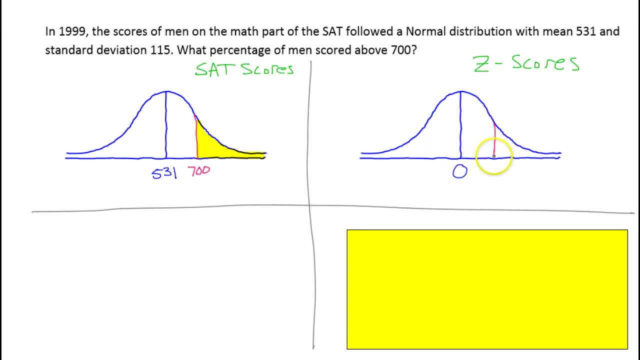 Okay, that corresponds to an SAT score of 700.. We need to find out what that z-score is. Okay, we need to figure that out, And whatever it is, then somehow we need to find the percentage of data to the right of it. 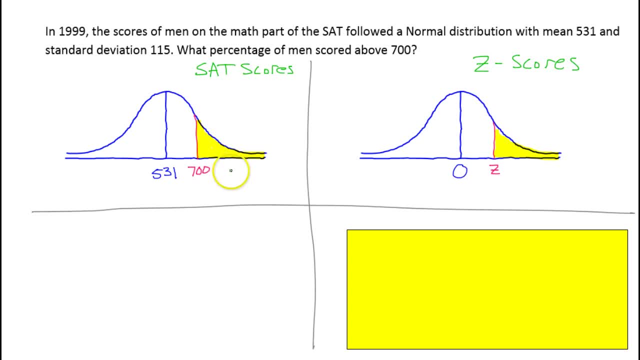 Okay now the first step is very easy. We can find the z-score that corresponds to a 700 SAT score. In other words, we can convert this SAT score to a z-score. Now the formula goes like this: If you want the z-score, 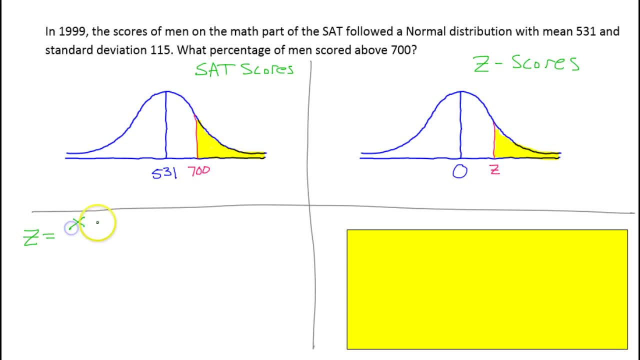 uh, what you do is you take whatever value you have, you know, like this 700, and you subtract it from, you subtract the mean from it, and then you divide by the standard deviation. So that is what I'm about to do. 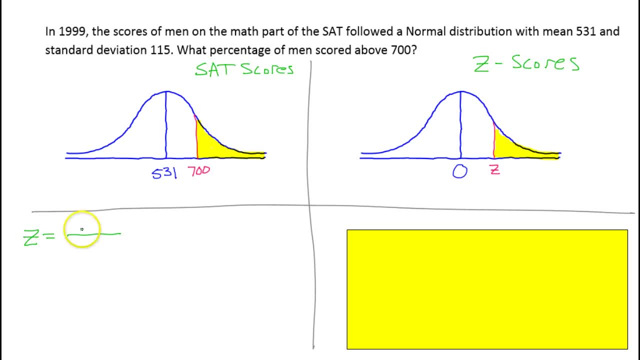 So I'm just going to replace these values with what I just said. So we're going to do the 700 minus the mean, which is 531, divided by the standard deviation, which is 115.. Okay, I'm just going to run. 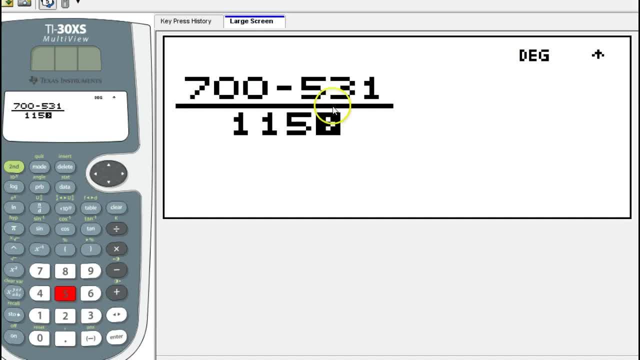 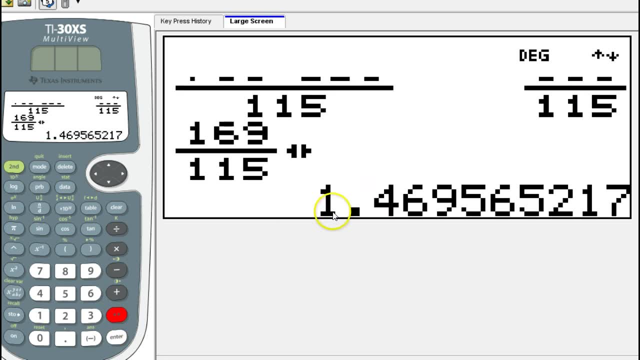 that through my calculator real quick. All right, so there you go. boom. Well, we really need decimals, so I'm going to toggle that Now. we're going to do two decimal places. It's very important that you round properly. 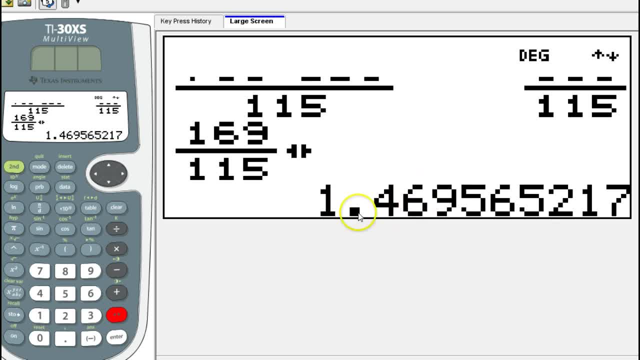 to the hundredths place. So I am not going to say 1.46, oh no, the next number is a nine, so I need to round up. all right, If the next number is five or higher, you got to round up. 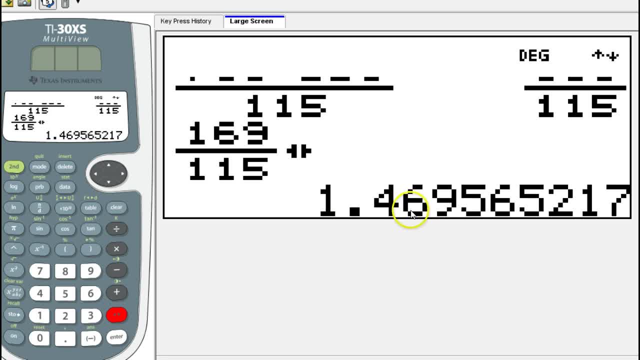 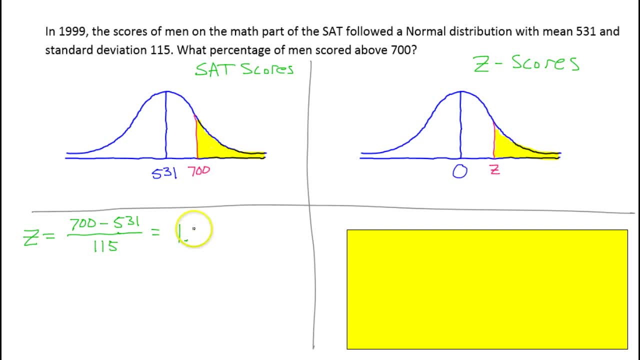 So this is going to round to 1.47.. Okay, so what I have here is a z score of 1.47.. So that is this value right here. Okay, 1.47.. Okay, this means it's almost one. 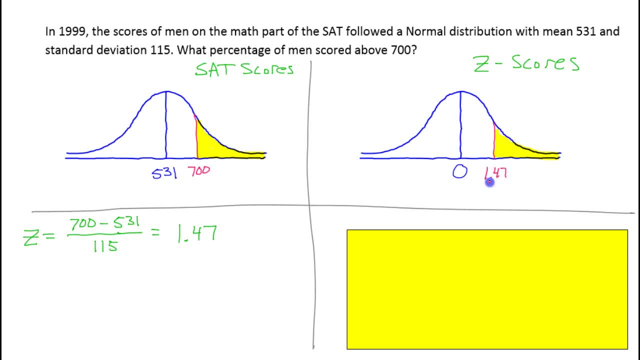 and a half standard deviations above the mean. That's what 1.5 would be. one and a half, All right, the z score is how many standard deviations above the mean you are. Anyway, now here's the problem: We've got the z score. 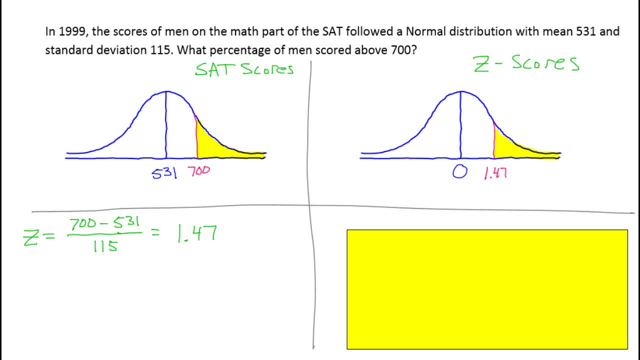 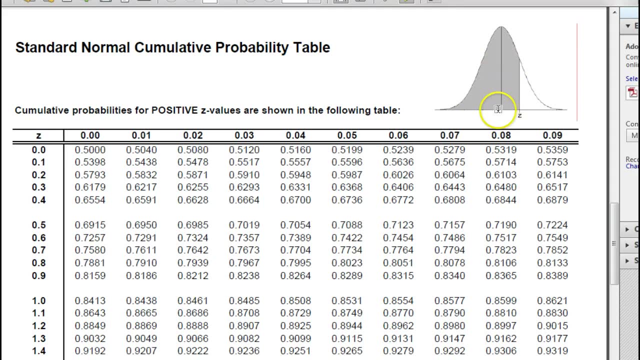 We want to know what percentage of the data is above the z score and we've got this chart. The only problem is this chart, and you can tell by this little diagram here, sort of reminding us. this chart tells us the percentage of data below any given z score, not above all right. 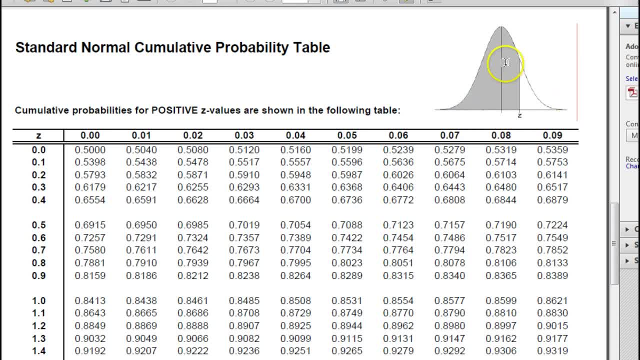 So, for example, if this part over here below the z score is 60 percent, how could we find what percentage of the data is above this z score? Well, we could subtract from 100,. all right, If the left side is 60 percent, the other side must be 40 percent. 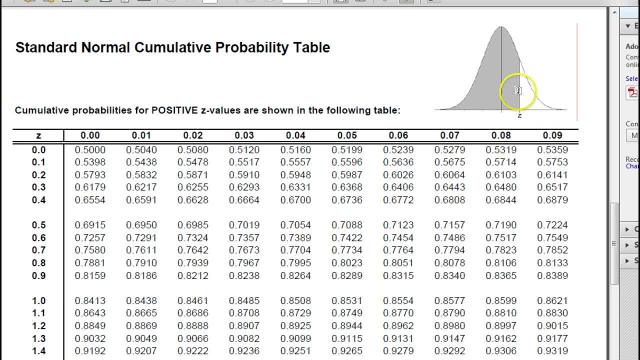 It all has to add up to 100. So just understand. this chart is going to give you the percentage of the data that is to the left of the z score, below the z score, If you want the percentage of data that's to the right. 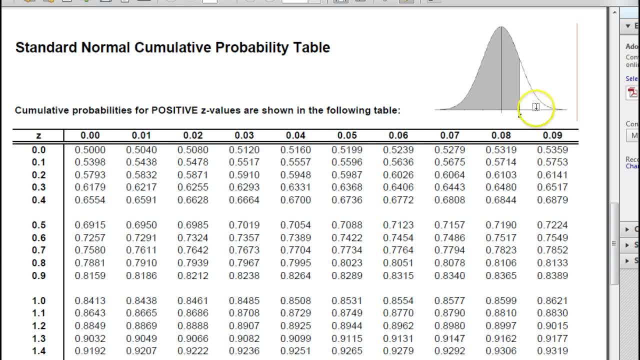 or above the z score, you're going to have to subtract from 100, okay, If this is 80, then this will be 20, you know that type of thing. So that's what we're going to have to do here. 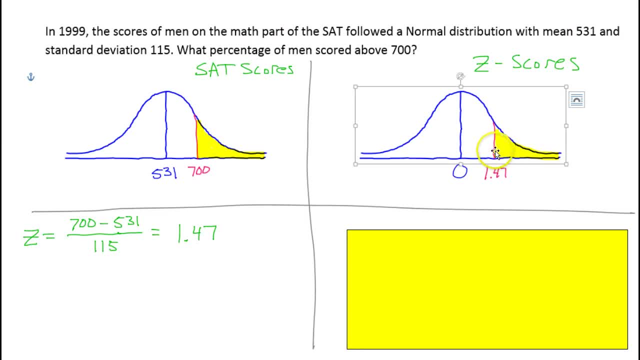 because we do want the percent of the data that is above, So we're going to have to subtract from 100.. Okay, and here's how you could write this as we continue our calculations: The percentage of z scores that are quote-unquote: 80 percent. 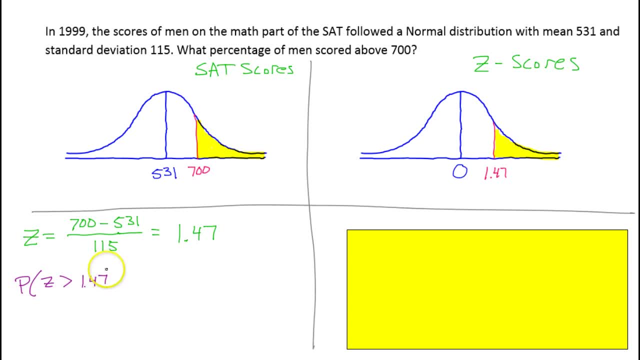 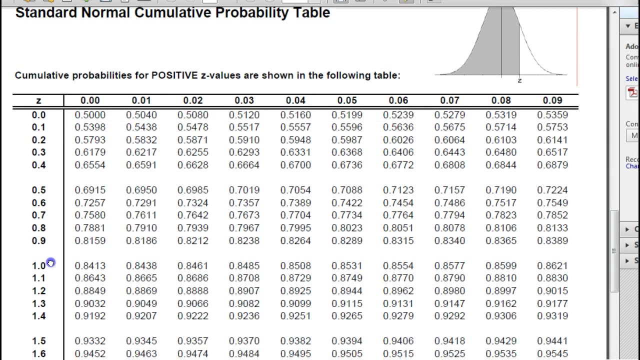 greater than 1.47, that's going to be 100 percent minus whatever we find on the table. So let's find 1.47 on the chart And here's how you do it. okay, Here's 1.4, it's going to be this row. 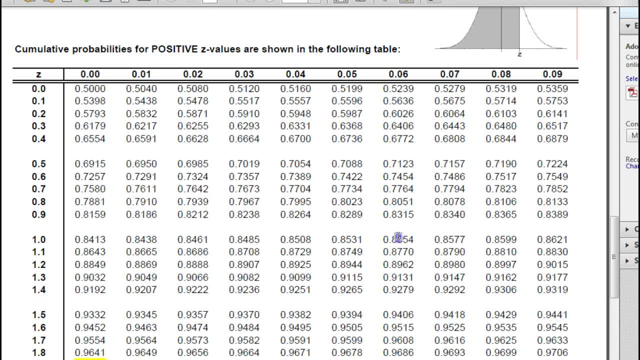 Now the 7 tells us exactly which number to look at. okay, So we start at 0, and then it's 0.1234567.. All right, so put that together. So 1.47, is this number, right there? 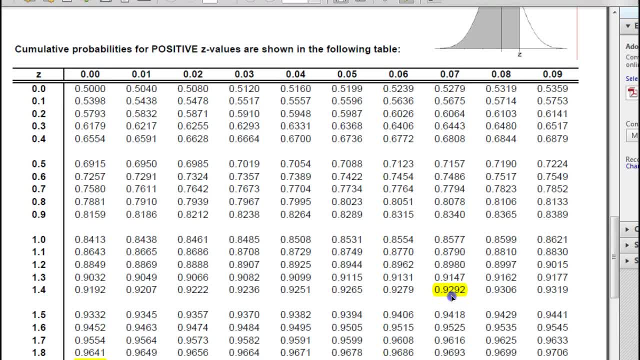 All right. so this means 92.92 percent. Now remember, that's the percentage of the data that's to the left of that z score. If we want the percentage of data to the right, we have to subtract from 100.. 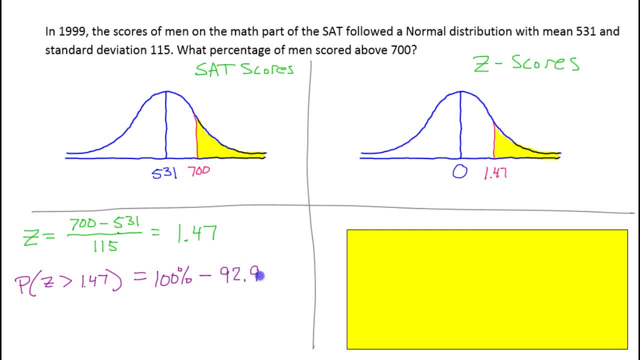 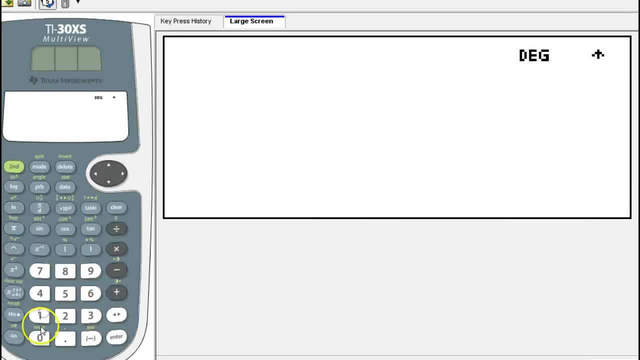 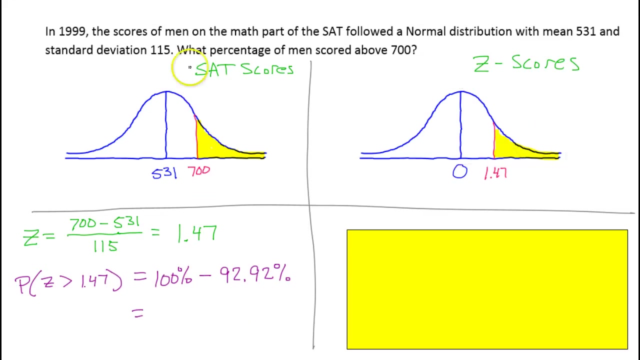 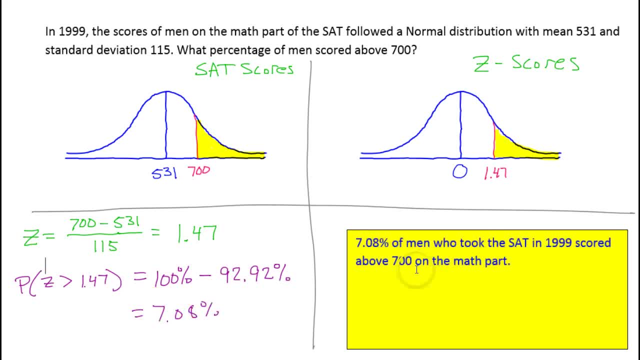 Okay, so that is 7.08.. All right, in the last section here we summarize the answer in a sentence, because this is a real-world problem, so we don't want to just spit out a number. We want a sentence that captures the context of the situation. 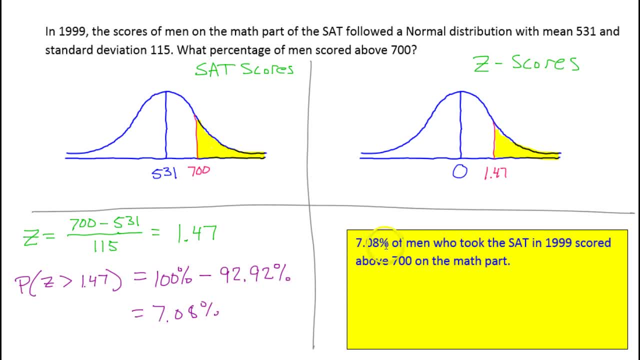 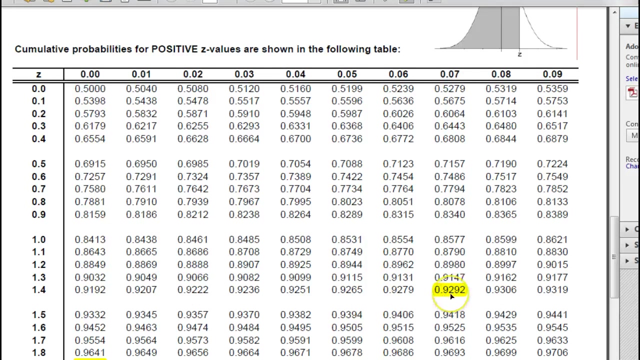 So 7.08 percent of men who took the SAT in 1999 scored above 700 on the math part. So that's the answer. Let me just say one more thing here. So remember, off the chart we saw the 92 point, you know. 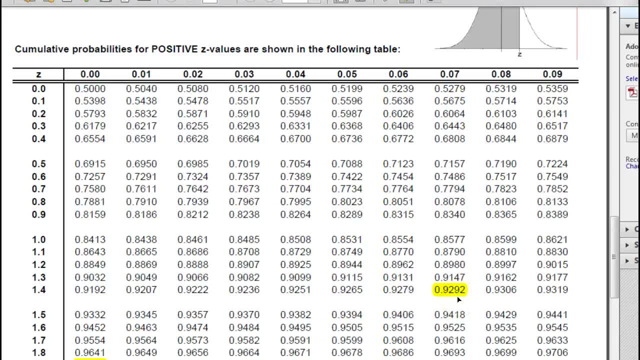 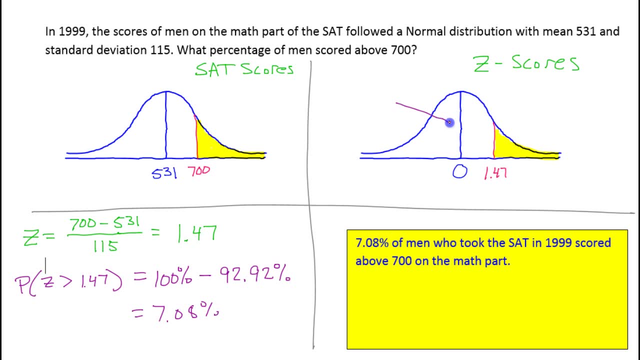 the .9292, which translates into 92.92 percent. I told you that that number is the percentage to the left of the z score. Okay, so I just want to just emphasize this to you. This left side of the graph here. 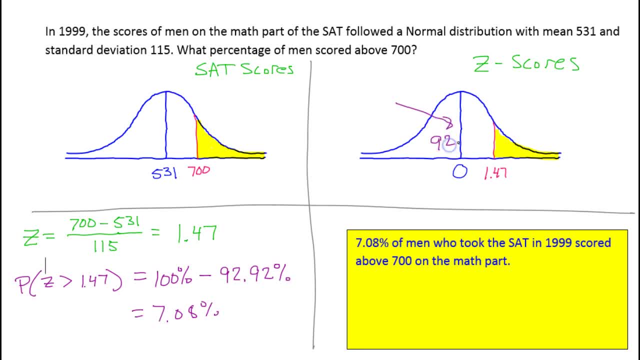 the white side represents 92.9,. I can't write today 2 percent. That's the white side here, And then the left side here. the yellow side is the 7.08 percent. Okay, This number, all right, see, I mean that's just. 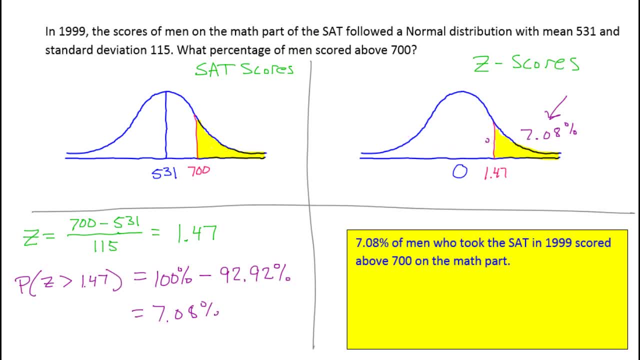 let me see if I can do a better job of writing that number. So this side with the 92.92 percent is the white side. That's the number we read off the chart. It's always going to be the left side If we want this side to the right- the 7.08,. 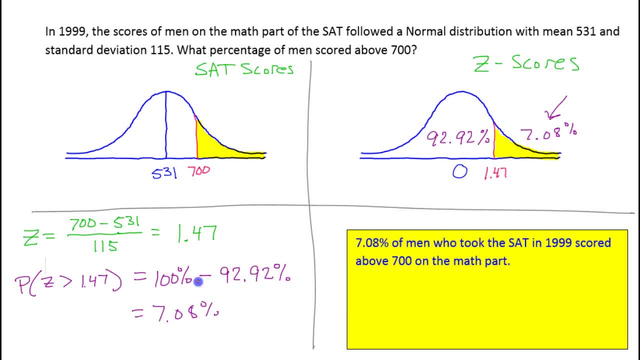 remember we had to subtract from 100. If the question had said what percentage of men scored below 700, then we would not have subtracted from 100. The answer would have been: 92.92 percent of men scored below 700. 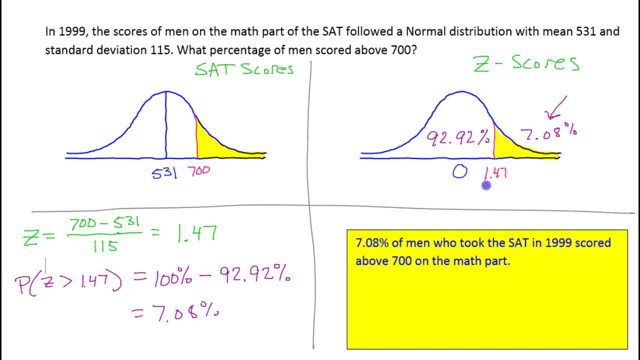 Oh, by the way, I mean I keep. I'm talking about these percents and I'm saying above and below 700, even though here we have the z score of 1.47.. I should say this, you know out loud, I guess. 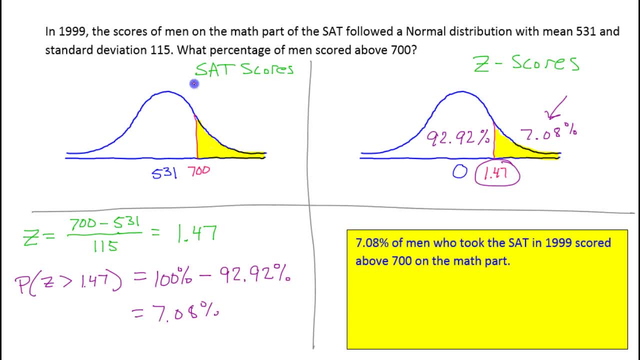 The thing is, the reason why we have the z score picture, the z score picture and the SAT score picture- is that the percentages are the same. Okay, So fine, we found the percent of z scores that are to the left of this number.